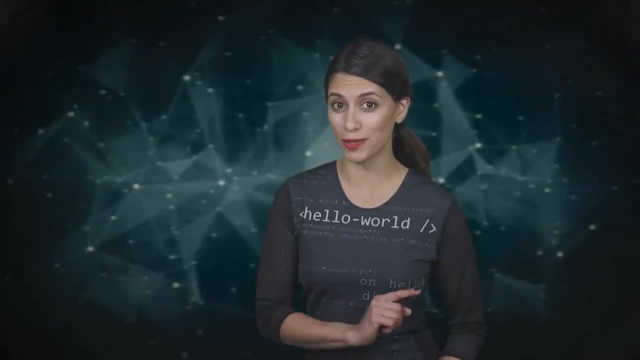 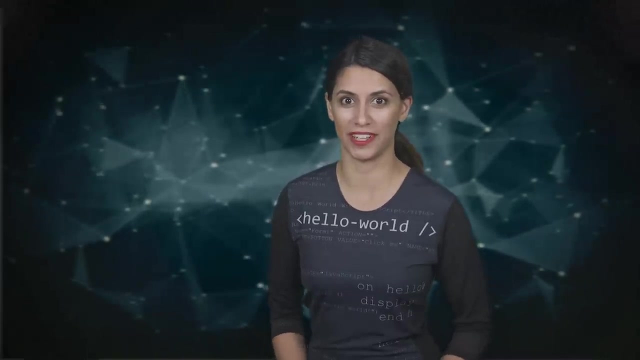 It's true, You can use a computer to do work, but you can also use a computer to have fun. Wow, Really, You can use it to do your math, homework or draw a picture or go on the internet. We send emails using computers. I'm talking to you right now on a computer, using video chat. 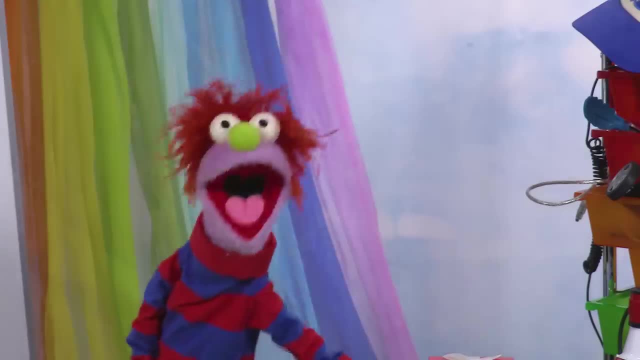 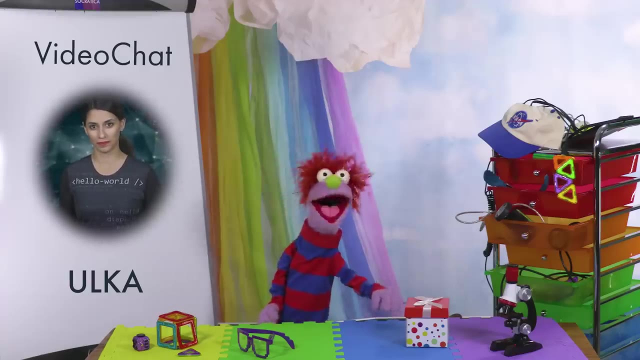 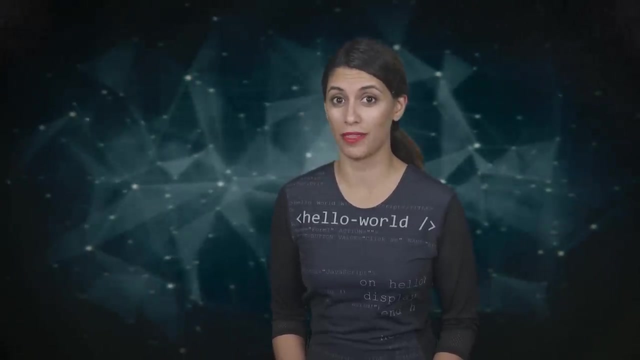 Gosh, Computers must be very, very smart. They're only as smart as their software, That's the instructions that tell the computer what to do. Which part is the software? Can you point to it? No, I can't point to the software. All the parts you see, that's the hardware. 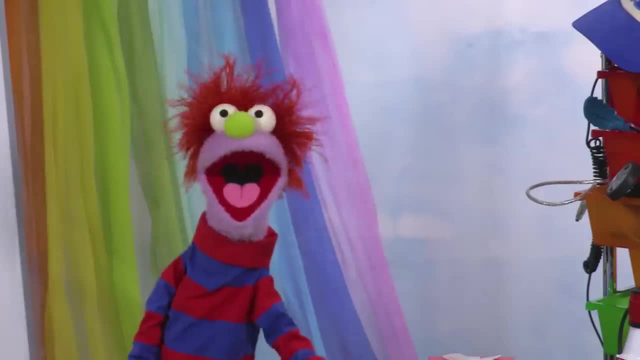 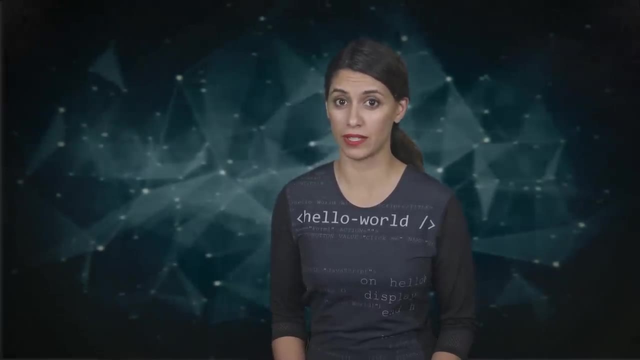 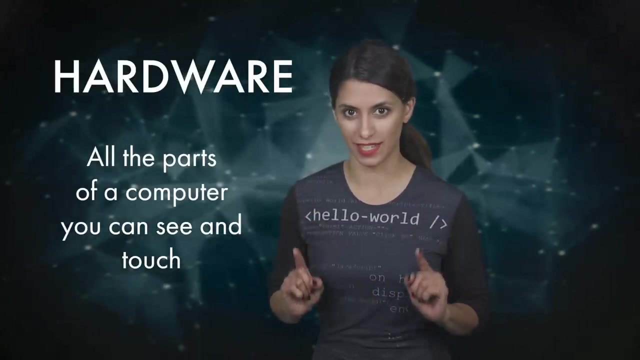 Hardware and software. That's a good joke, Tony Uka. I'm actually being completely serious. Computers work by combining hardware and software. Hardware is anything physical, anything you can see and touch, Like the monitor, the keyboard and all the parts inside the computer. 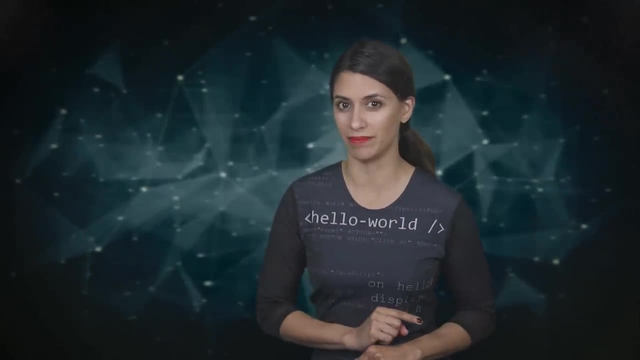 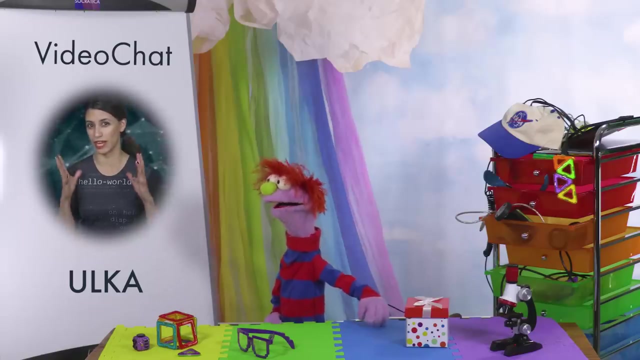 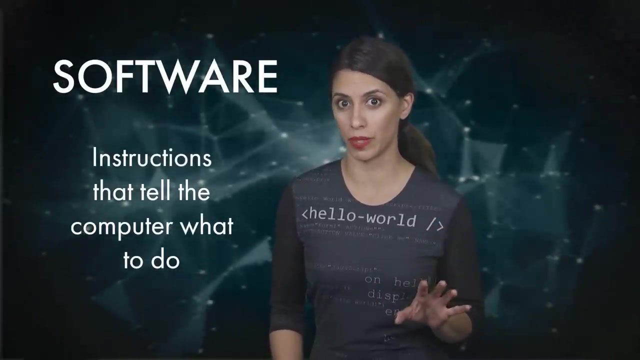 All those wires and circuits. That's where the real work gets done. On this circuit board you'll find a computer CPU, the central processing unit That's like the computer's brain. Oh, So what do you mean by software? Software is the set of instructions that tell the computer what to do. 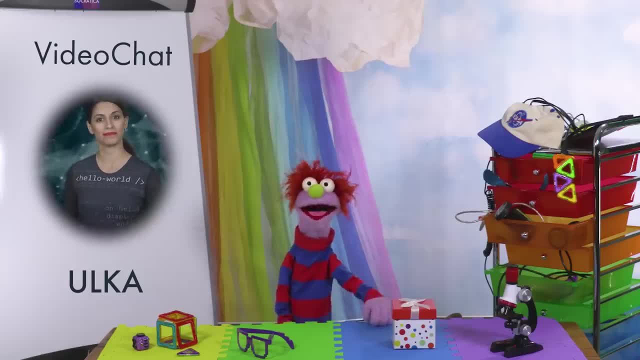 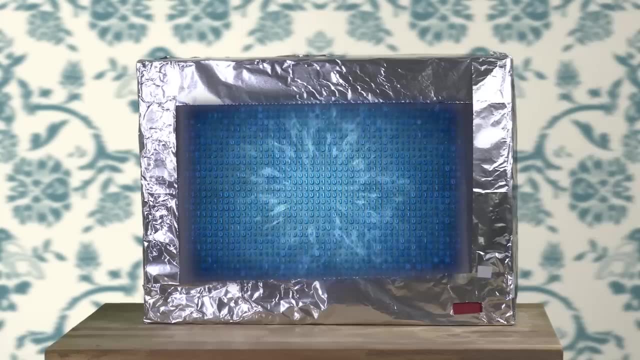 That's where we come in. We do, Yes, Your computer doesn't have any idea what it's doing. In fact, it won't do anything at all ever, unless you tell it to. Wow, That's a lot of power. 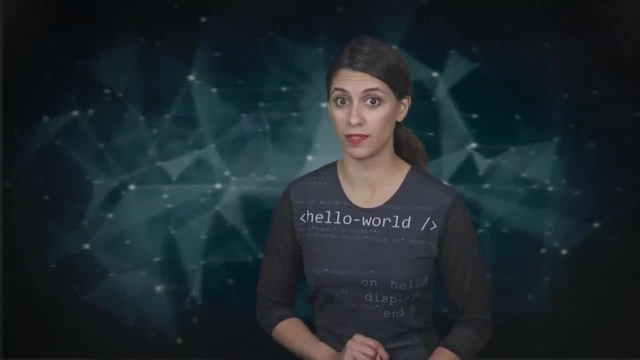 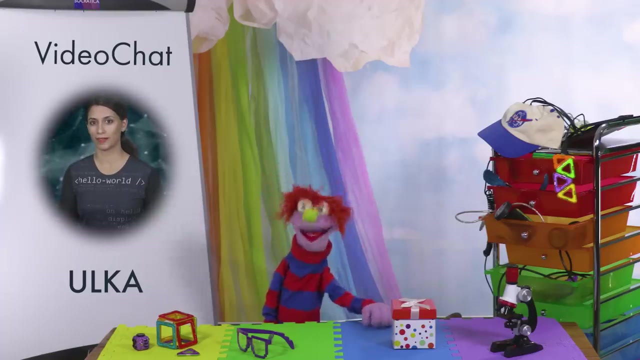 Yes, You need to be very careful about what kinds of instructions you give your computer, or it won't work properly. Oh Well, how hard can it be? Would you like to try to write very careful, step-by-step instructions like how a computer needs them? 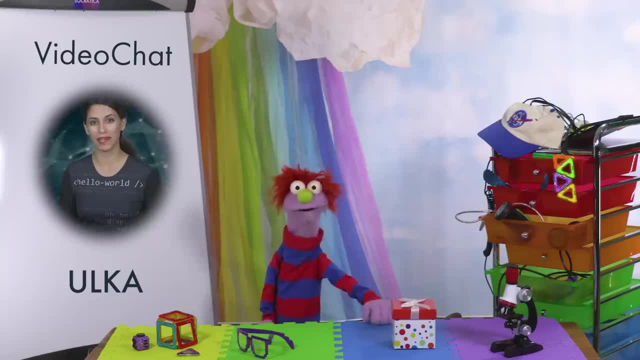 Sure, sure, sure, sure, I got it, I got it. Then let's make a peanut butter sandwich. Oh, I know how to do that. I make myself peanut butter sandwiches as a snack, sometimes after school. Good, Then this should be very easy for you, right? 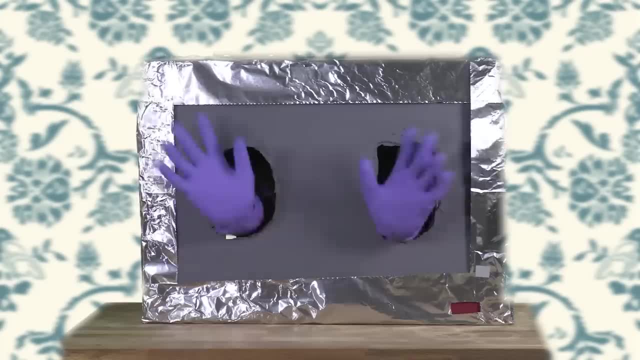 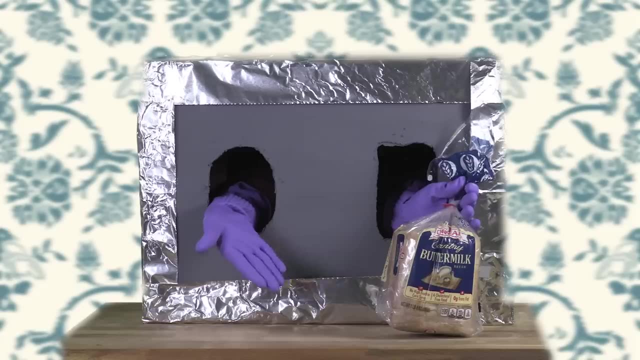 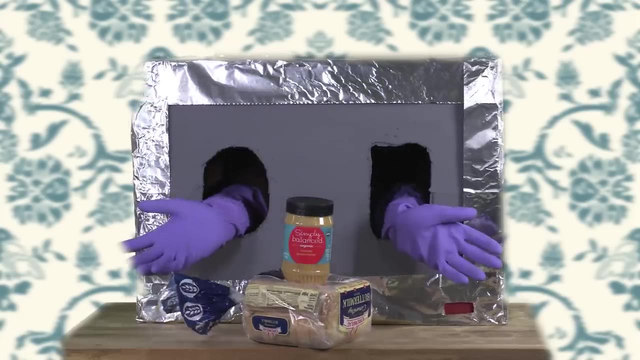 Right, Pretend your computer has hands. How would you tell it to make a peanut butter sandwich? Well, you'd tell it take some bread and some peanut butter and you put the peanut butter on the bread Like this. No, That's silly. 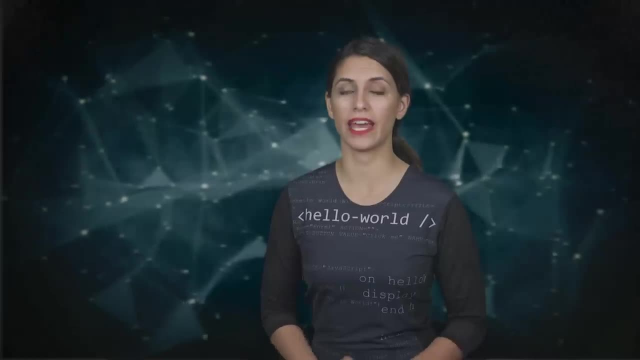 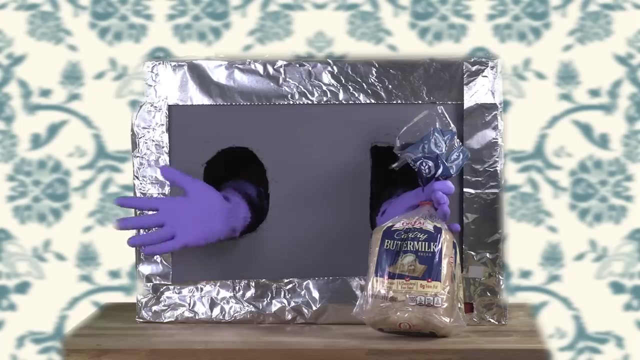 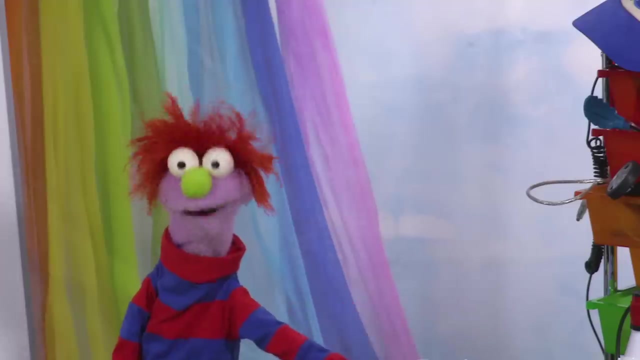 Well, the computer doesn't know that. You have to tell it everything step-by-step. Try again, Okay. okay, You take some bread. Wait, You open the bread and take two slices out. Now you take your peanut butter. 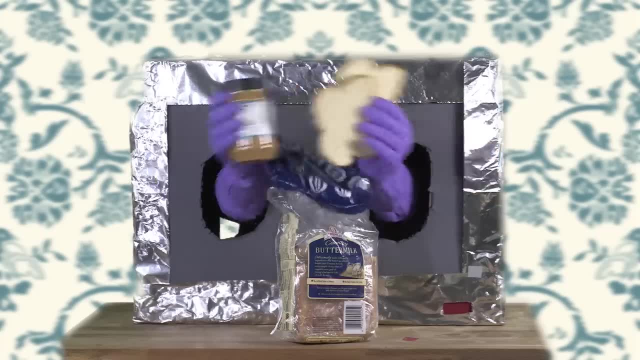 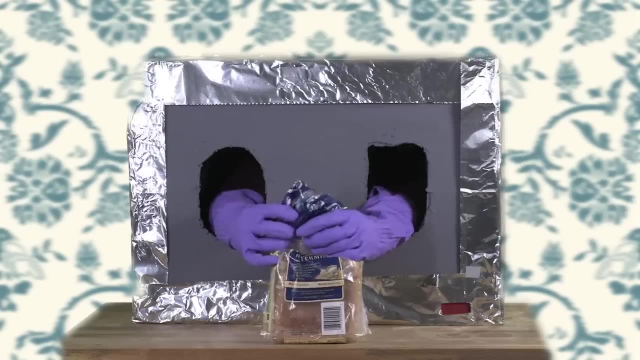 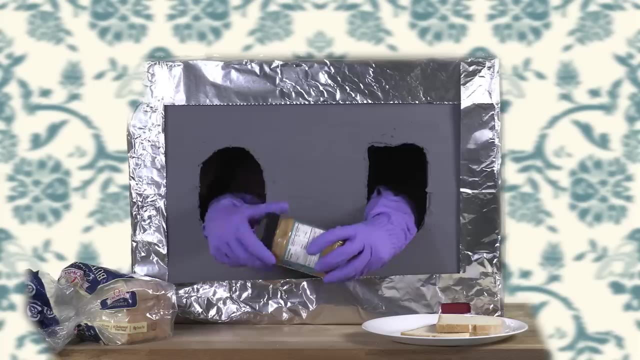 and put it on the bread Like this: Oh my gosh, Now let's start again. You open the bread. Take out two slices, Put them on a plate. Now open the jar of peanut butter, Stick a knife in. 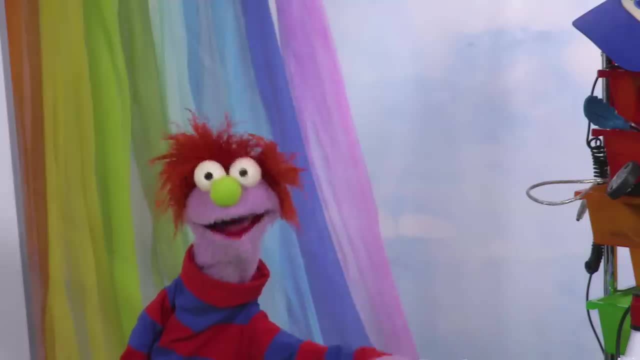 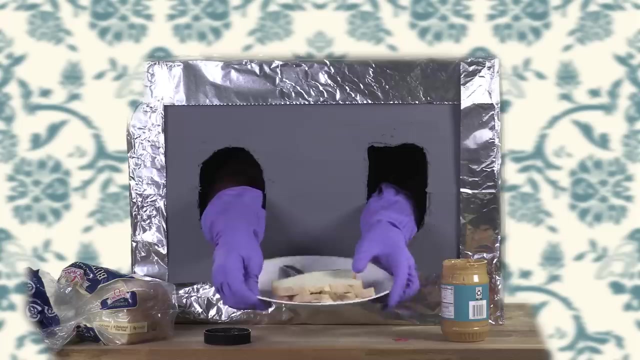 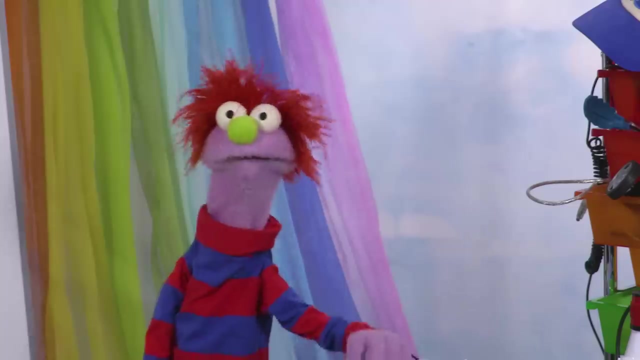 And use it to put the peanut butter on the bread. Bleh, Bleh, Stick the two pieces of bread together. Mmm, Looks like a pretty crunchy sandwich there. Oh my gosh, One more time, Open the bread. 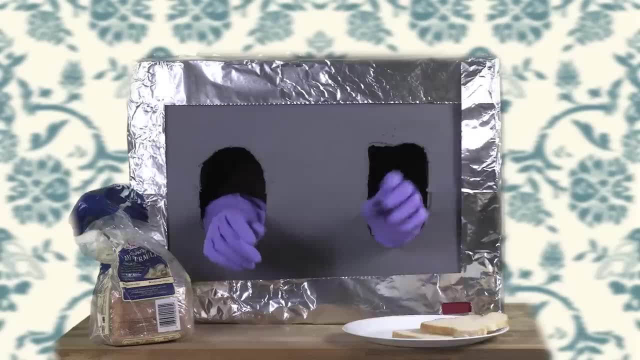 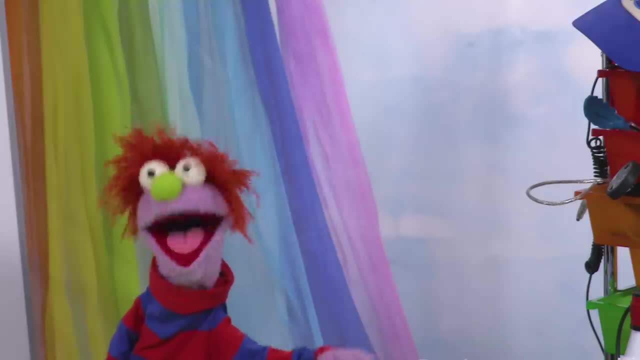 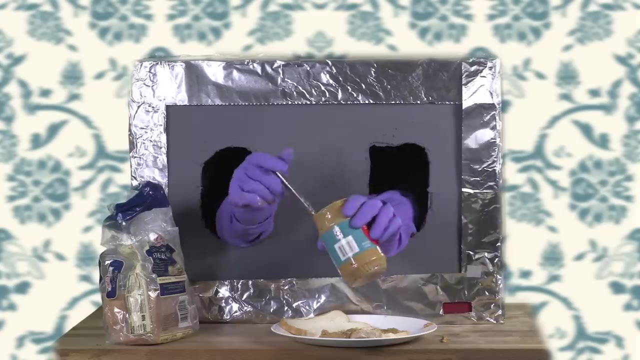 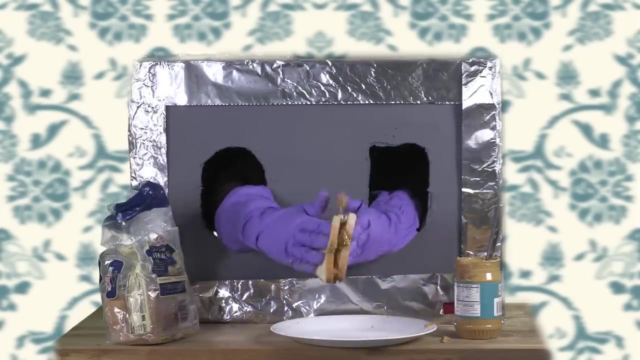 Take out two slices. Put them on a plate. Open the jar of peanut butter. Stick in a knife. Use the knife to spread peanut butter on the bread slices. Put away the knife. Close the two pieces of bread together. Okay, that looks like a pretty good sandwich. 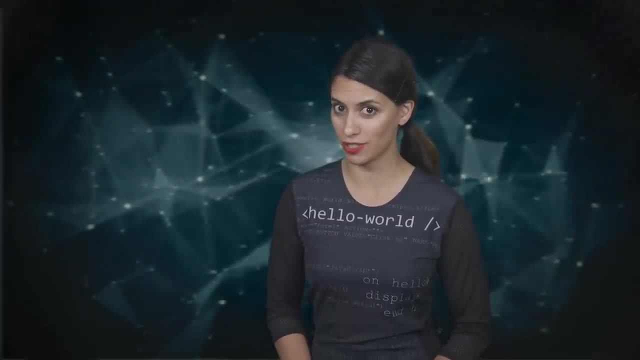 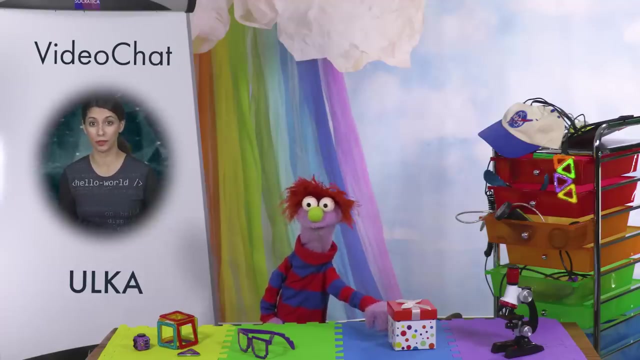 Now do you see what I mean about having to be very careful with your instructions? Yes, That's what software is: The step-by-step instructions you give your computer. One set of instructions is called a program. You just wrote a peanut butter sandwich program. 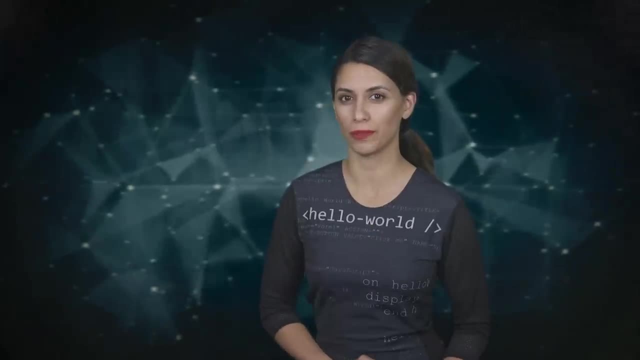 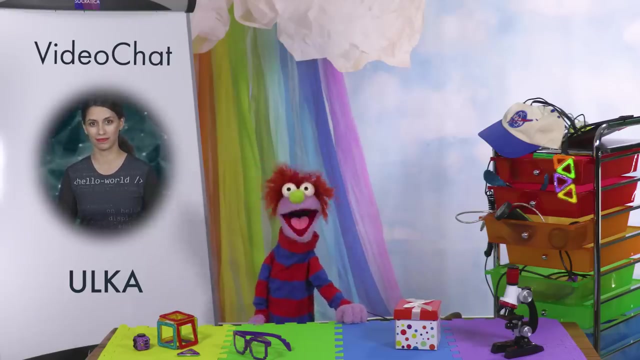 I think I could get the hang of this. One more thing, Topher. We've been speaking English to your computer, But computers actually speak different languages Like French. Non mon petit chou, Computers speak computer languages. For example: